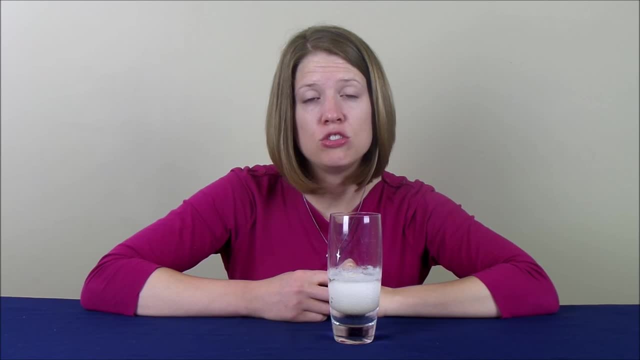 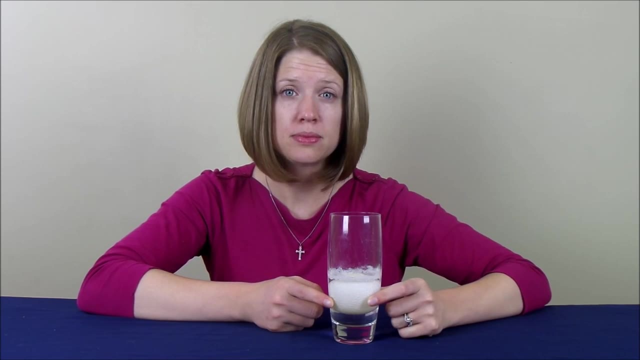 So it has been 3 days since we put the egg into the vinegar, so let's check in on it. So the first thing you're going to notice is the egg itself is swollen. The other thing you'll notice is there are still a lot of bubbles around the egg itself, And also if 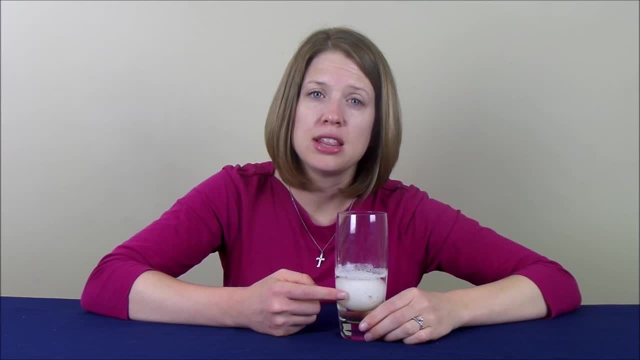 you turn the egg or turn the glass and you can take a look at the place on the egg where it's been rubbing up against the glass itself. it has started to turn translucent in color. So at this point we are ready to take the egg out of the vinegar and rinse it underneath. 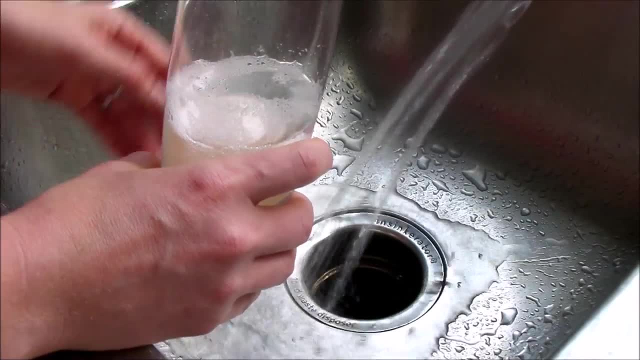 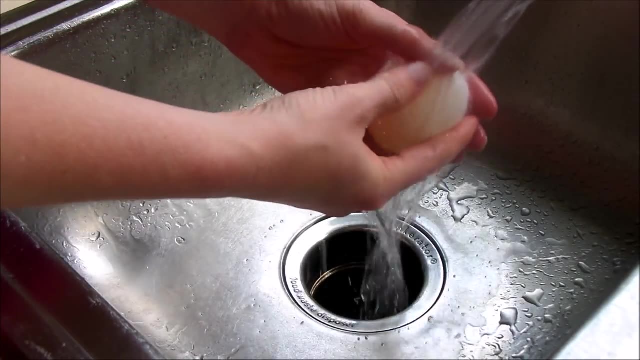 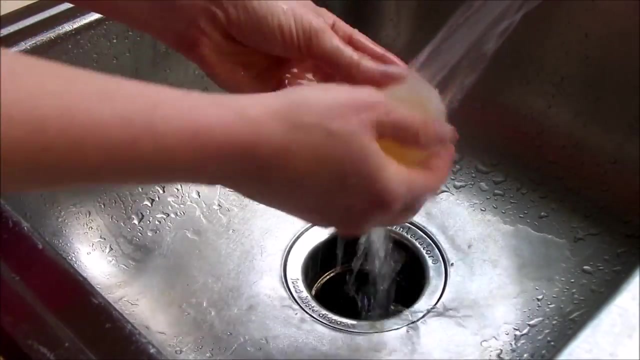 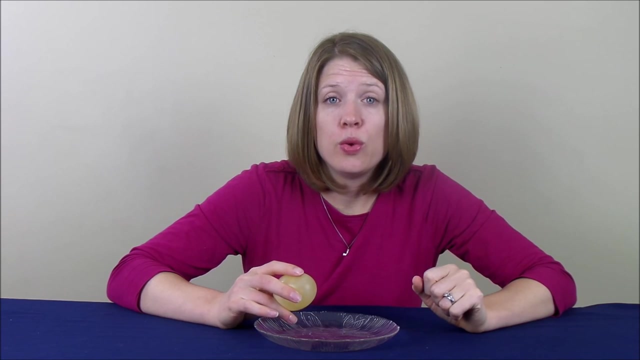 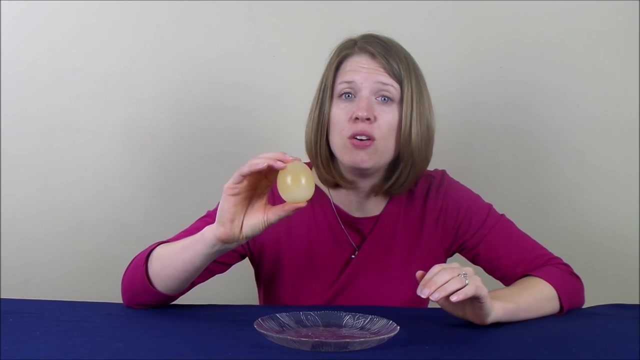 some tap water. So, as you noticed, when I was rinsing the egg under the water, I was gently rubbing the outside of it to remove the white film that was left on the egg. So now the egg is entirely translucent in color. 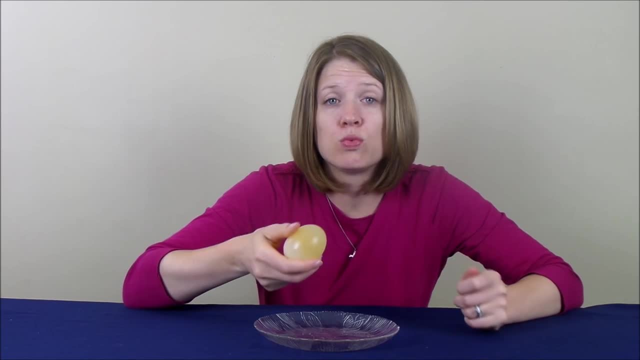 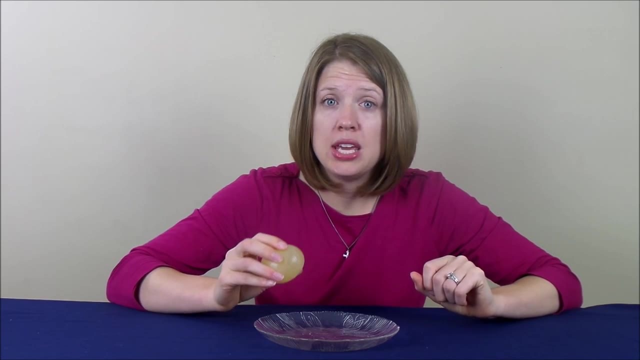 You'll also notice that when you squeeze it it kind of feels rubbery like a bouncy ball. So now let's see if it bounces. And when we do this we're going to want to keep it kind of low to the area that we're bouncing it. We don't want to drop it from too high of. 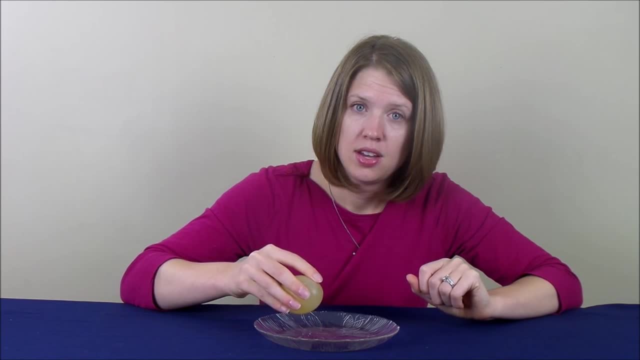 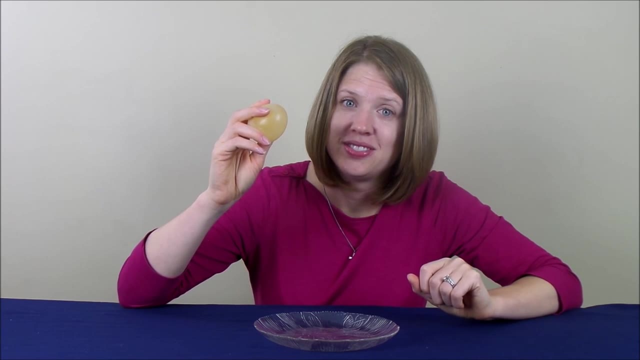 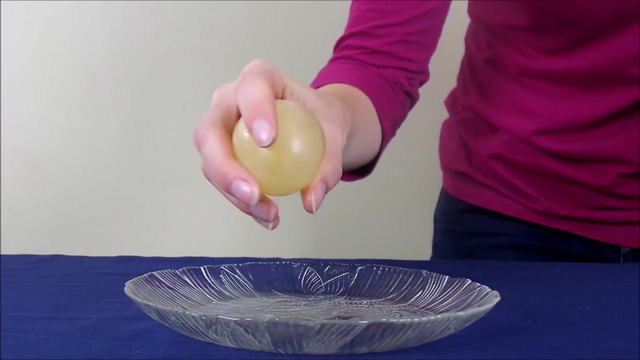 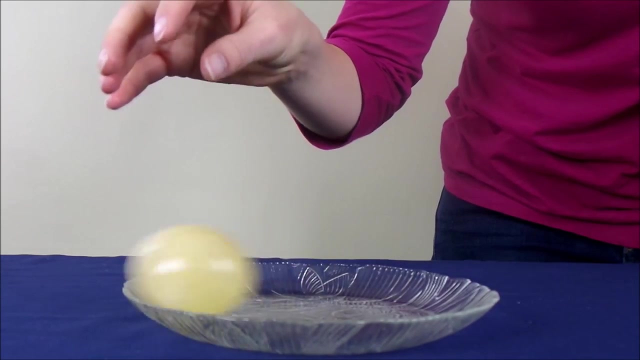 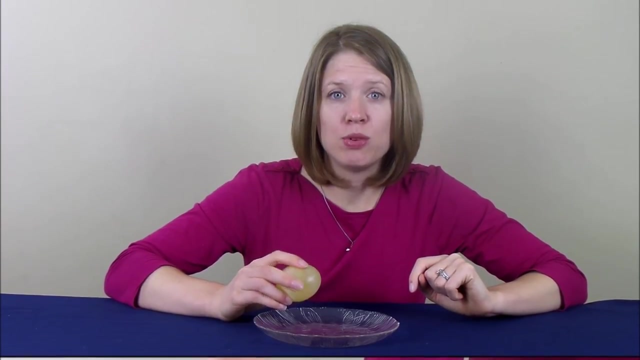 a height. Now do you want to know what happens when you do drop it from a high height? Be sure to watch to the end of the video. So let's bounce some more. Do you know how we were able to turn a raw egg into a bouncing egg? Leave a comment below. 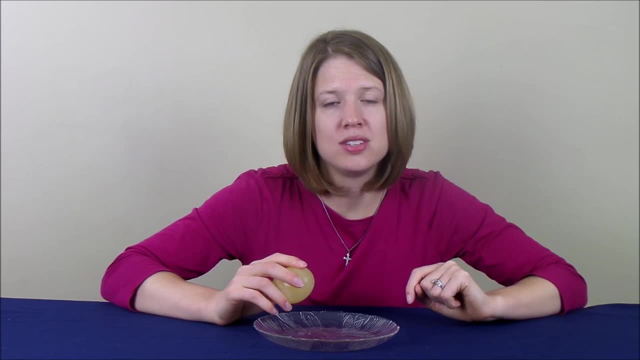 to submit your guess and then visit CoolScienceExperimentsHeadquarterscom to find out the answer. You'll be able to print out instructions for this video. I hope you enjoyed this video and I'll see you in the next one. Bye. 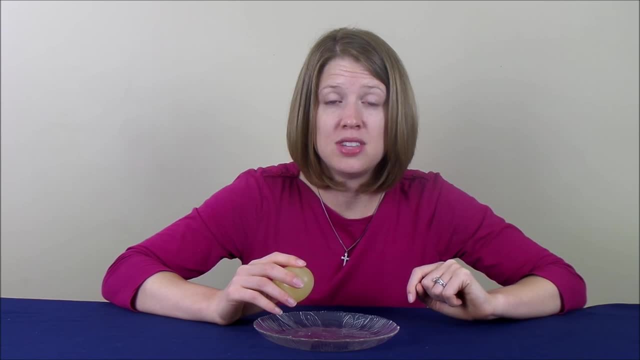 Thanks for watching everyone. We'll see you next time.